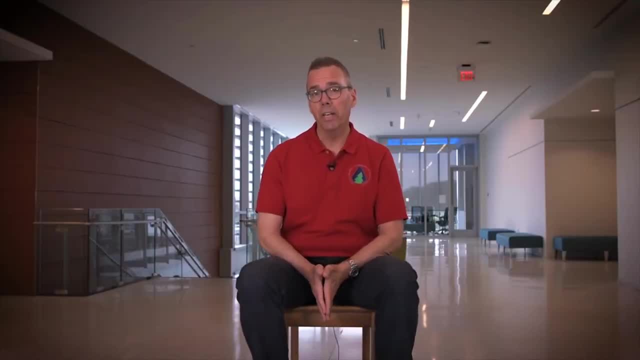 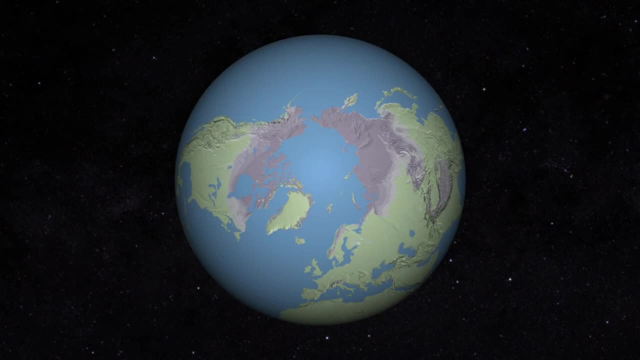 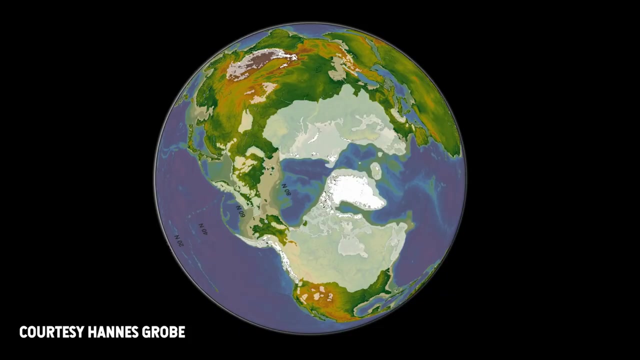 Permafrost is the hidden cryosphere. It's the permanently frozen soil that surrounds the Arctic. all across Alaska, northern Canada and then across Eurasia. The ground has been frozen during the ice ages. During the ice ages, there was not enough snowfall in the drier regions of Alaska. 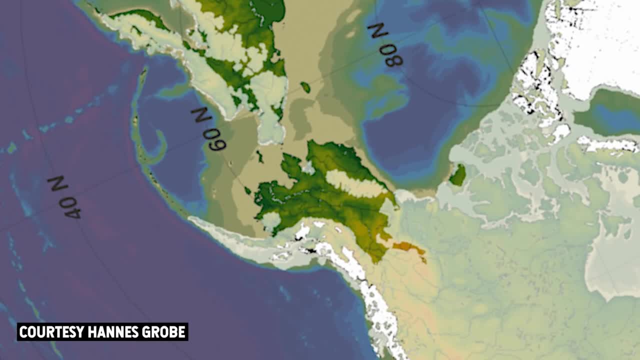 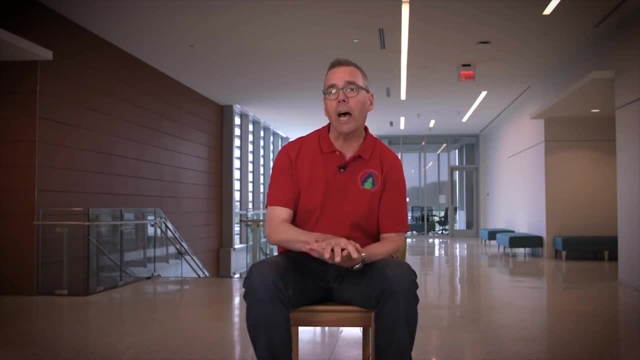 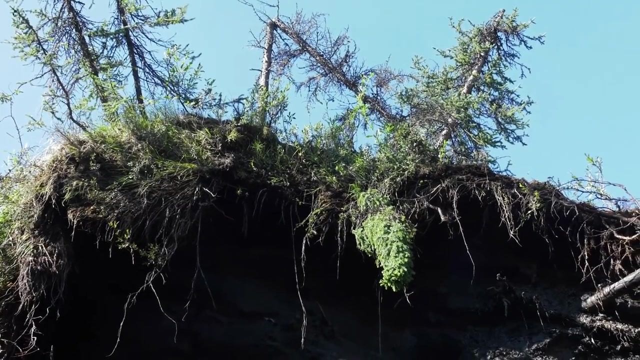 and Canada to form glaciers there, So the land was suitable for vegetation. What happened is that over thousands and thousands of years all of that plant material got compacted and frozen every winter and buried and pushed down so that today there's 300 feet deep. 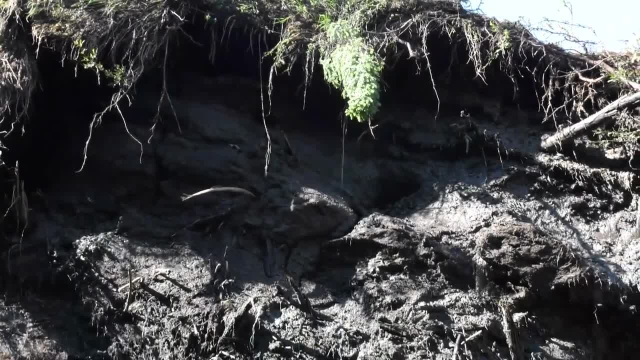 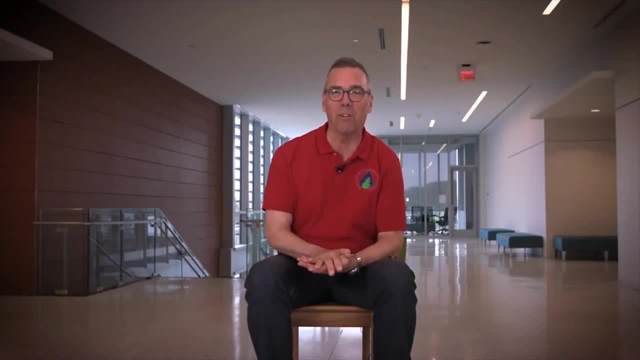 of frozen water and dead plants and some pieces of dead animals too. Sometimes you find woolly mammoths in the permafrost, But most of it, of the organic matter, as we call it, in the permafrost is frozen plant material. 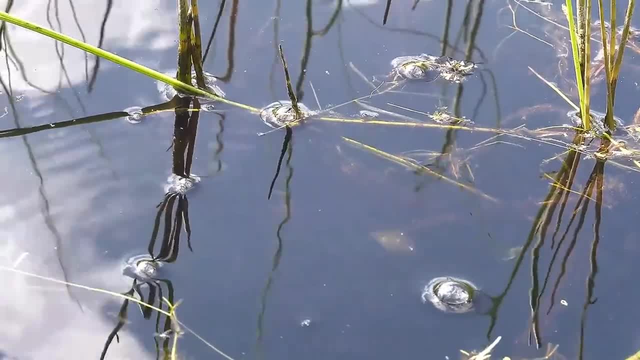 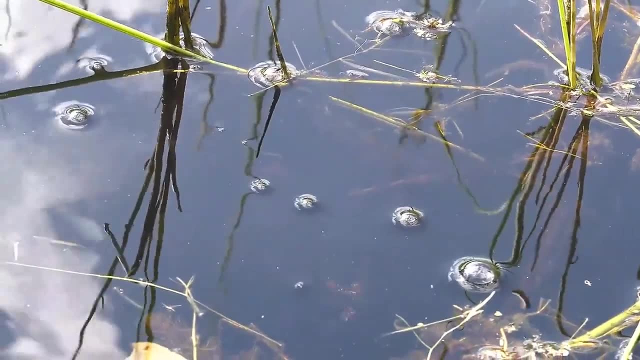 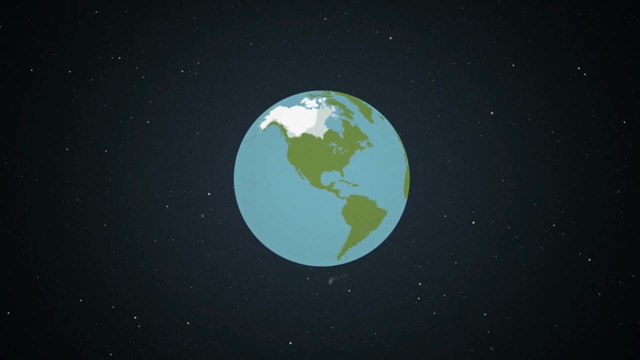 Some of that plant material is now thawing and decaying, releasing its ancient carbon into the atmosphere, sometimes in the form of methane gas bubbling out of expanding northern lakes. We started this field campaign because the Arctic is the part of the planet that is warming first and fastest. 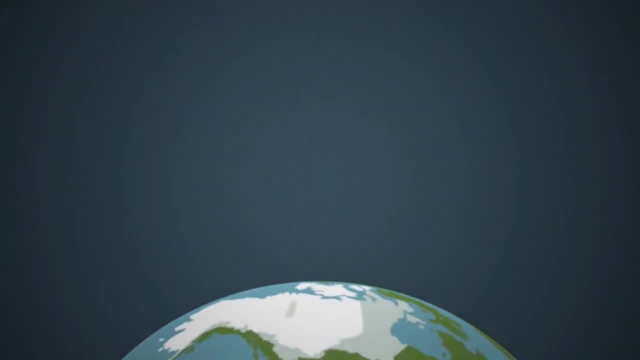 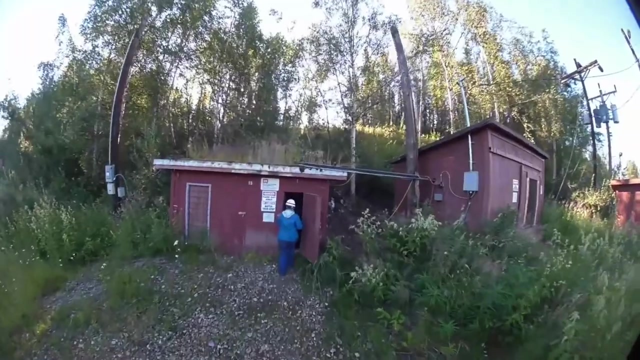 And there are consequences to this for permafrost. So during the Arctic Boreal Vulnerability Experiment, we're studying permafrost with people on the ground, from aircraft flying over the region and also from satellites in space- Another way to understand the permafrost. 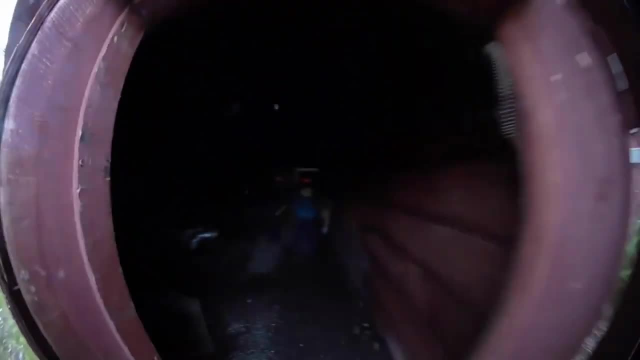 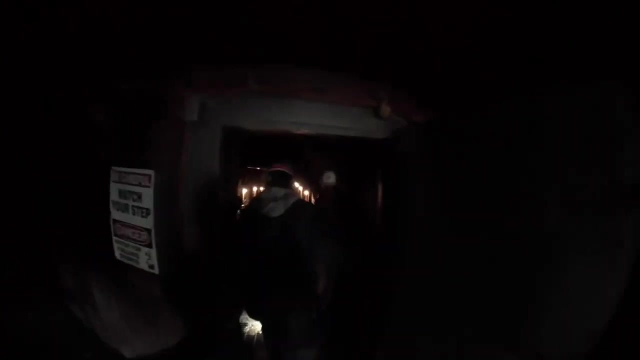 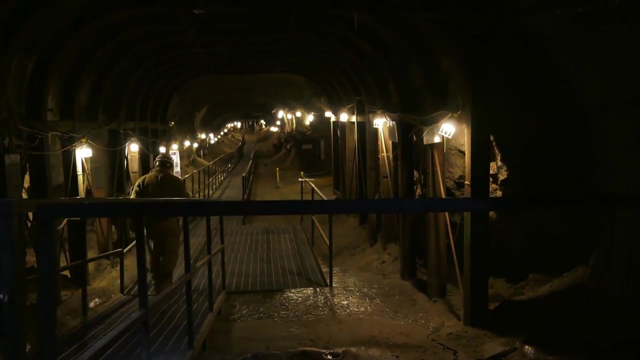 is to take a walk below ground with Matthew Sturm and into the US Army Corps of Engineers' permafrost tunnel. And they've dug this tunnel back into the side of a hill about 200 feet and it goes sort of sloping down. 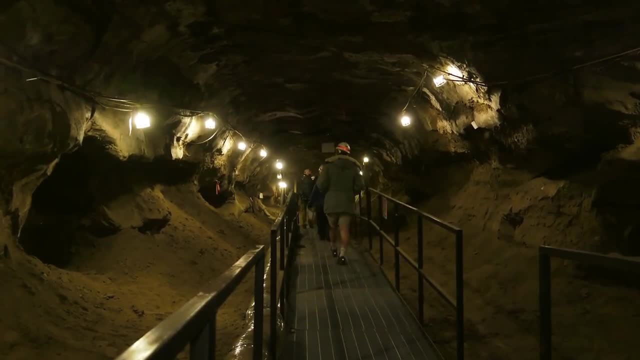 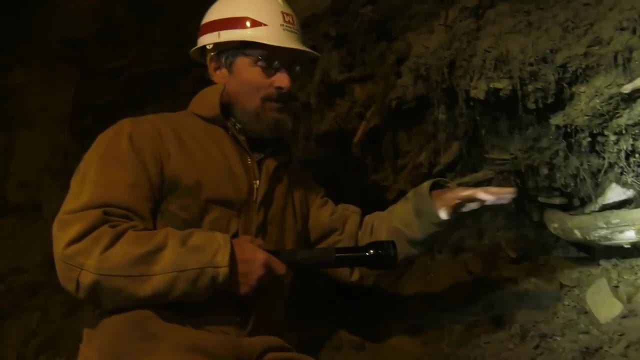 so that by the end of the tunnel you're about 100 feet underground And you're surrounded by bones sticking out of the wall from the steppe, bison and mastodons that are frozen in it. There's sticks that are 40,000 years old.